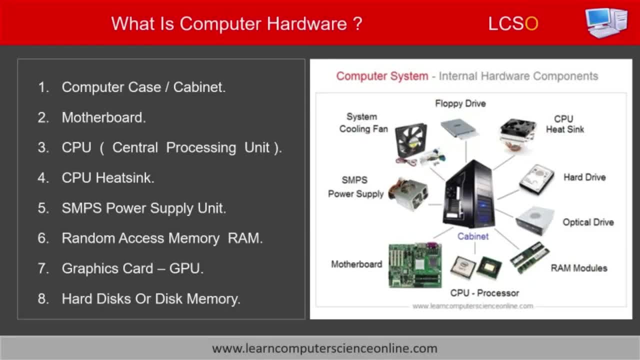 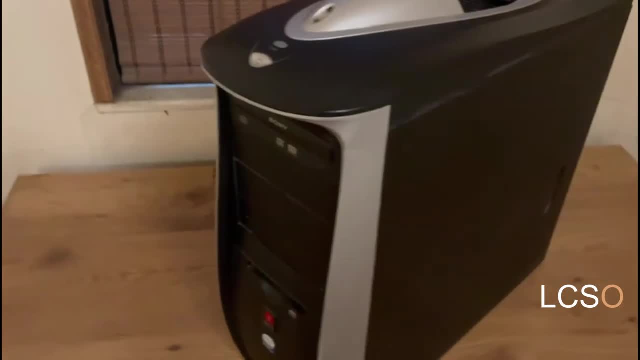 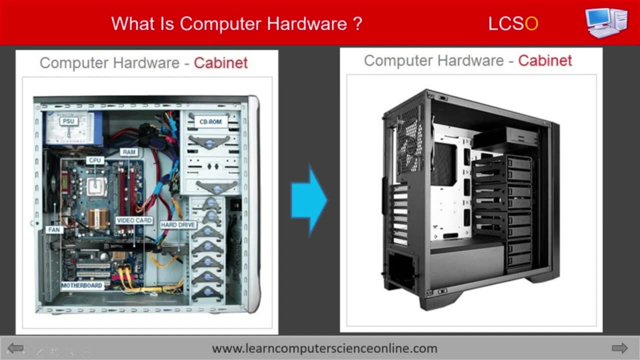 Let us start with the first hardware component on our list, That is, a computer case. A computer case is also alternately referred to as a computer cabinet. A computer case is type of metal enclosure used to assemble the various internal hardware components of the computer system. The main function of the computer case is to provide 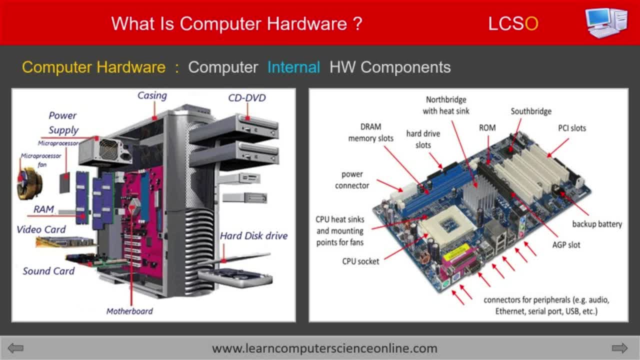 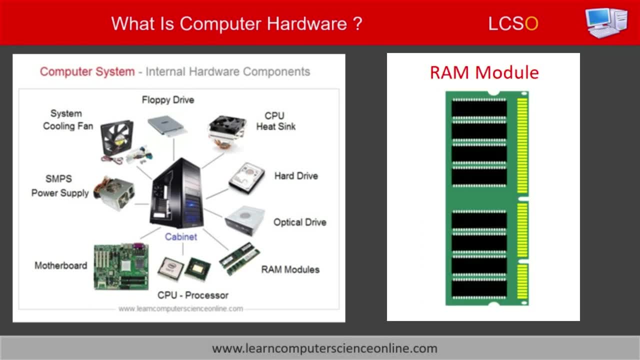 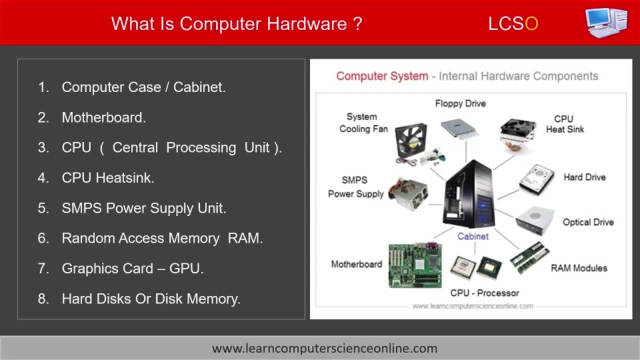 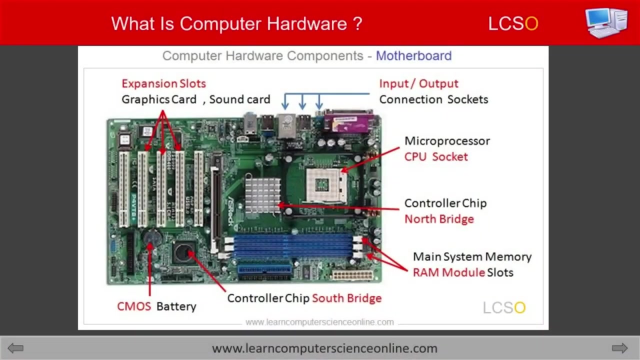 a protected enclosure to organize and assemble various internal hardware components, such as motherboard, microprocessor, data storage memory, hard disks, ram modules, smps, power unit and other such hardware components. let us move on to the next hardware component, that is, motherboard. computer motherboard is the main printed circuit board used to assemble and interconnect various 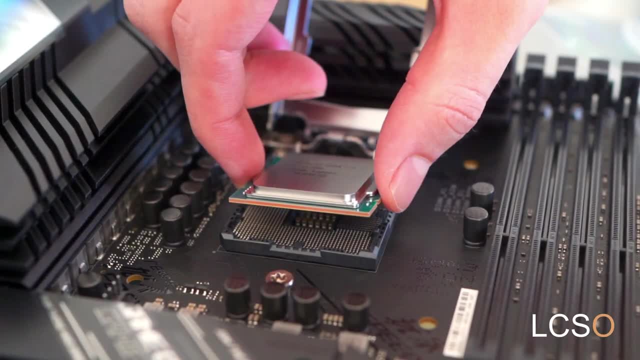 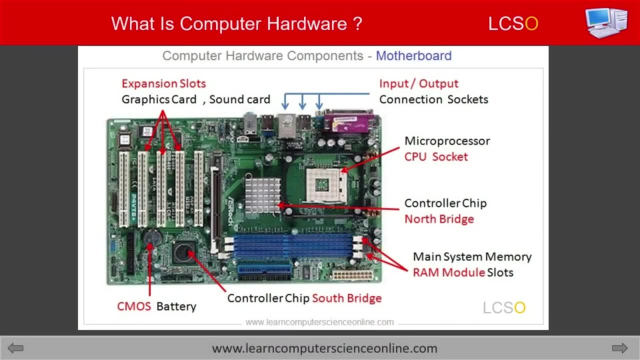 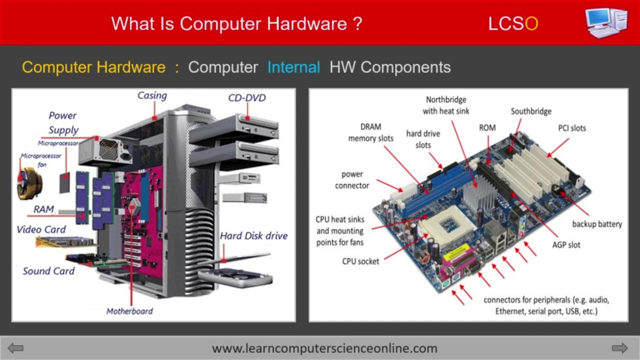 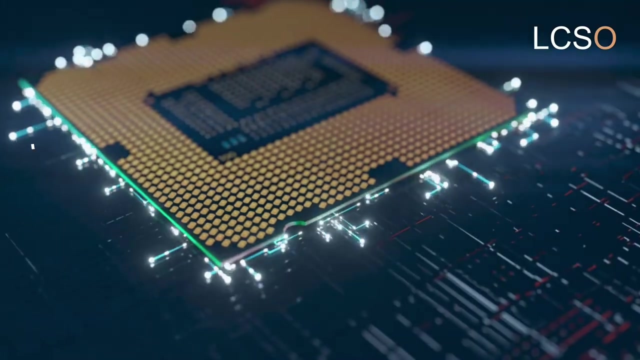 computer system components. the motherboard provides the connection sockets for the microprocessor, cpu, main memory, ram, secondary memory unit called hard disk graphics card, and the controller chips which connects the various input and output devices connected to the computer. the next hardware component on our list is called a microprocessor. microprocessor is the brain of 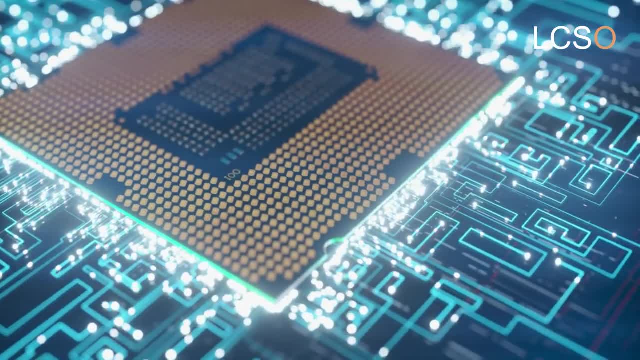 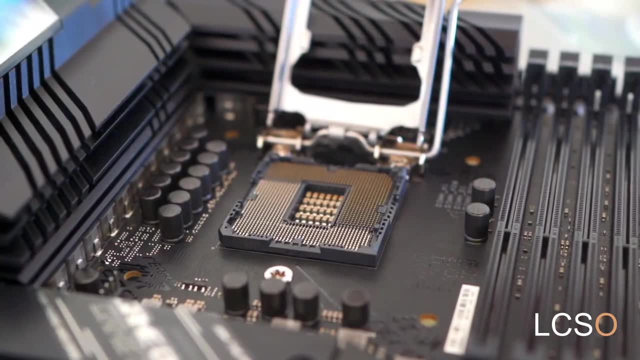 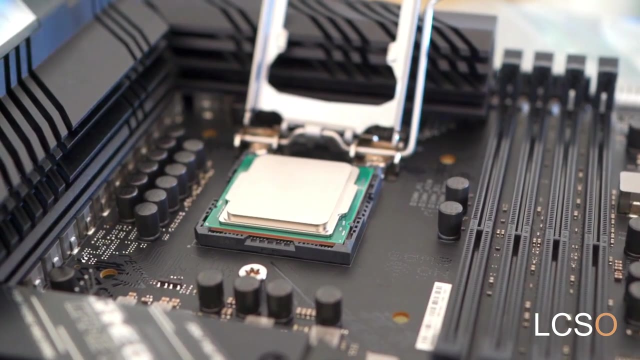 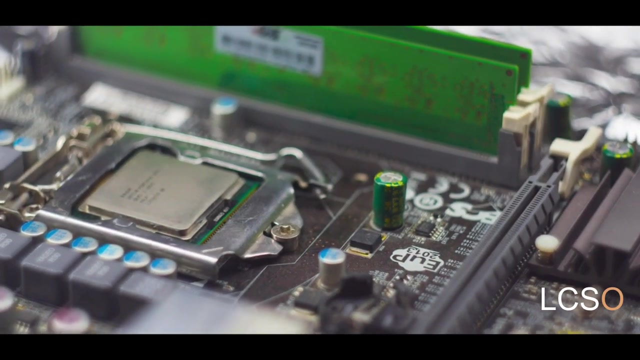 the computer system. it provides the processing power to the computer. the processor is also called as central processing unit, abbreviated as cpu. the microprocessor chip is mounted inside a special socket provided on the motherboard. the cpu socket is specially designed to firmly hold the microprocessor chip. with the help of its lever locking mechanism, the processor generates considerable heat. 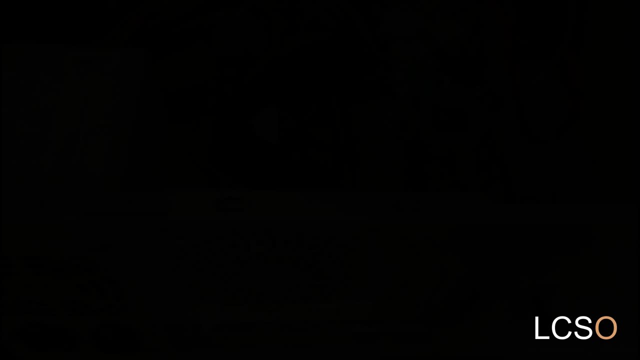 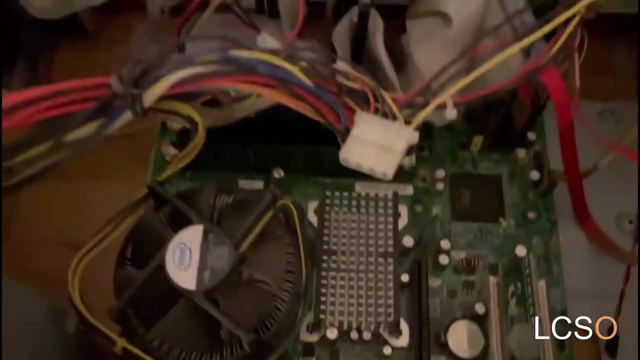 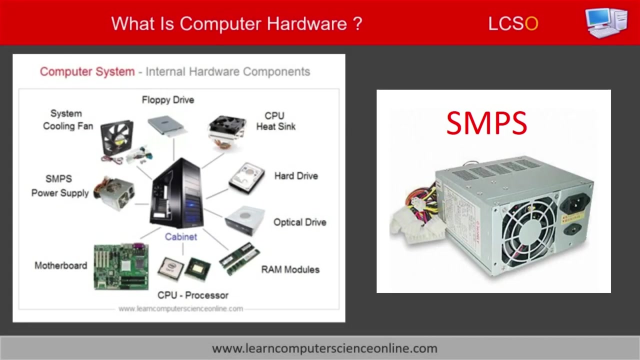 and therefore a special heat sink with miniature fan is placed on the top of the processor chip. this heat sink protects the processor chip from damage caused due to excessive heat. all right, let us move on to the next hardware component on our list, that is power supply unit called smps. the power supply unit is another important 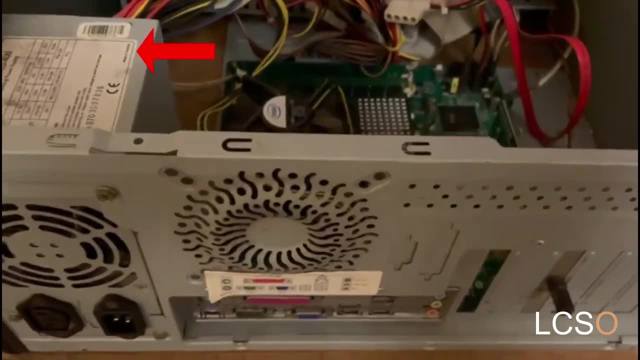 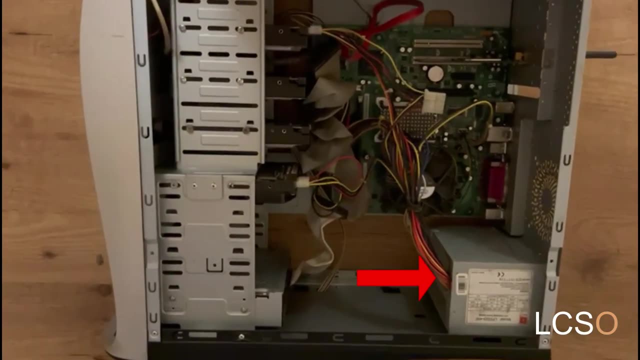 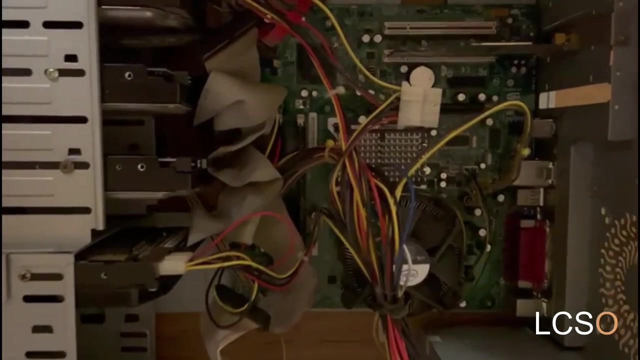 hardware component mounted inside the computer case. it is also called as switch mode power supply, abbreviated as smps. it is the most commonly used power supply unit that powers the computer. The main function of the power supply unit is to provide stable electrical power supply to the various hardware components present inside the 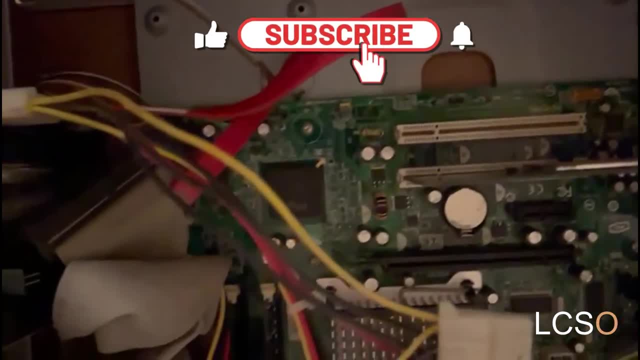 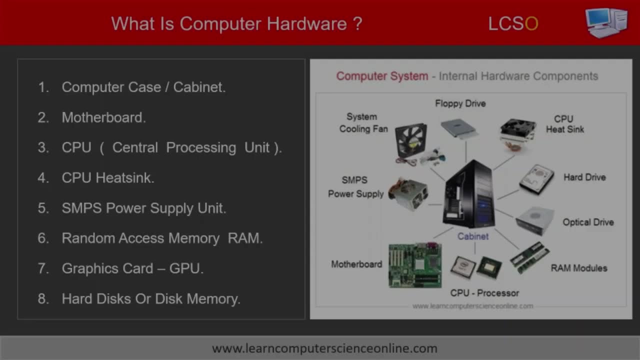 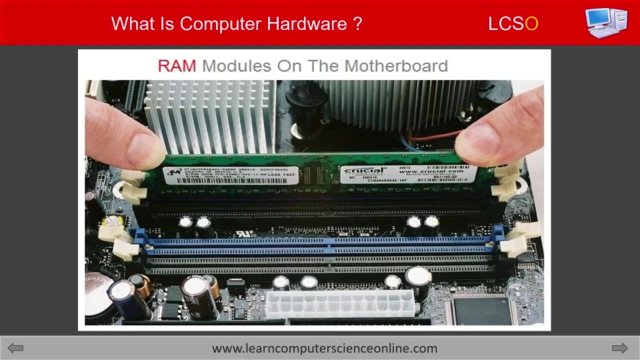 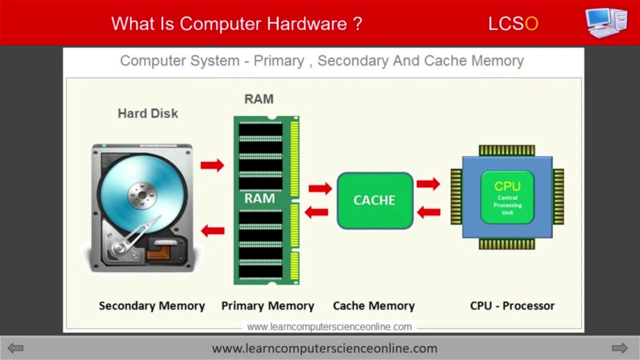 computer case. The SMPS unit provides multiple wire connectors to power different types of hardware components installed inside the computer case. Okay, let us move on to the next hardware component, that is, main memory, called random access memory RAM. The computer system memory unit consists of different types of memories organized in a hierarchical order with different 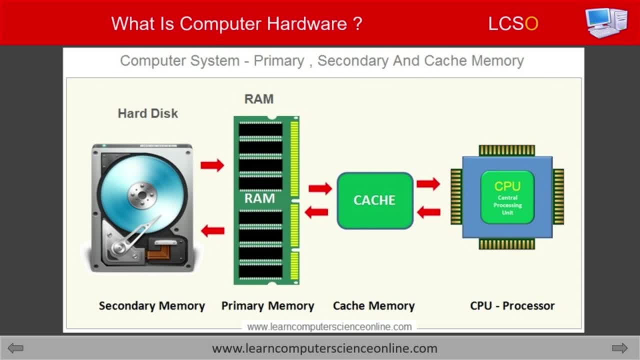 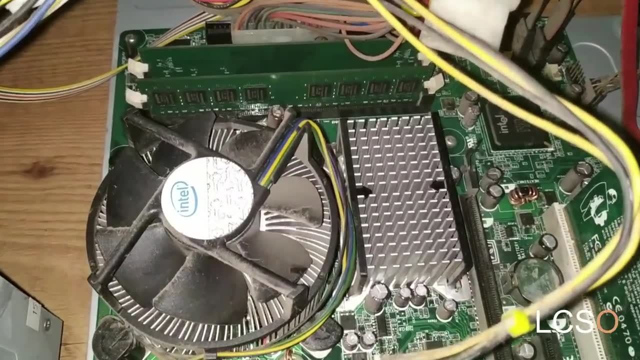 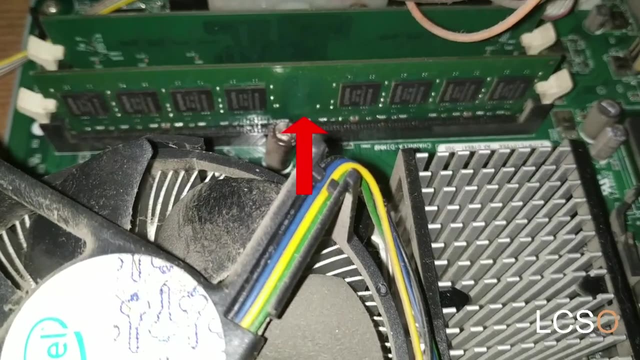 size and speed in order to optimize the system performance. Each of these memories performs a specific role during the program execution. The random access memory, RAM, is the main memory of the computer. The RAM is considered as a temporary or volatile memory of the computer because it can store the data till the time the computer is powered on. 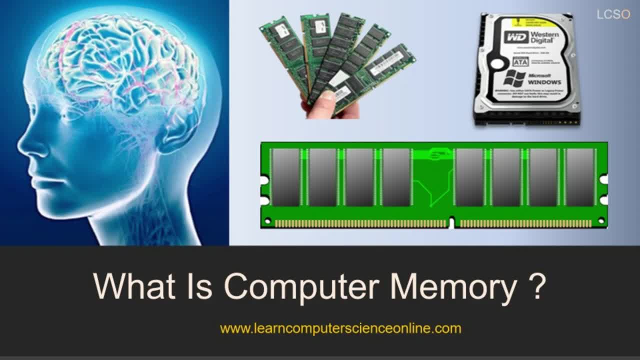 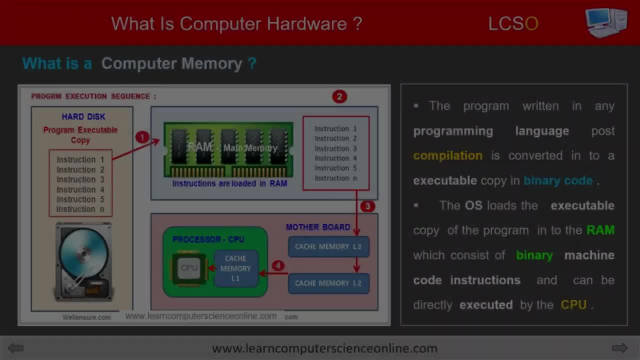 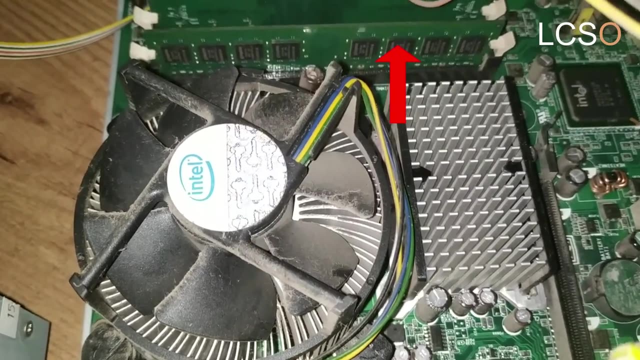 The main system memory, RAM, a critical resource that is managed by the operating system. The main memory is used to store the data and program instructions during the program execution. The main memory is present in the computer in the form of RAM modules installed on the computer. 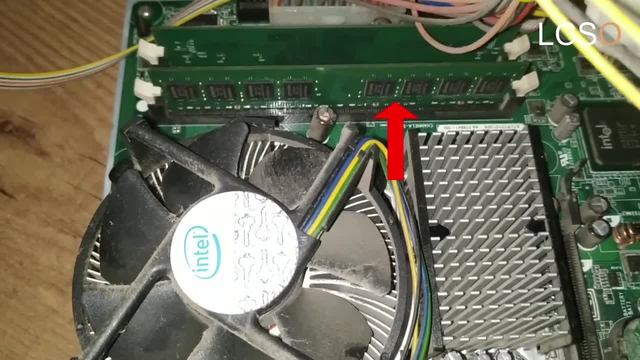 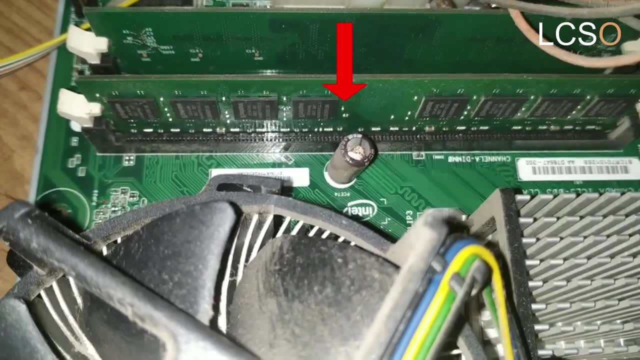 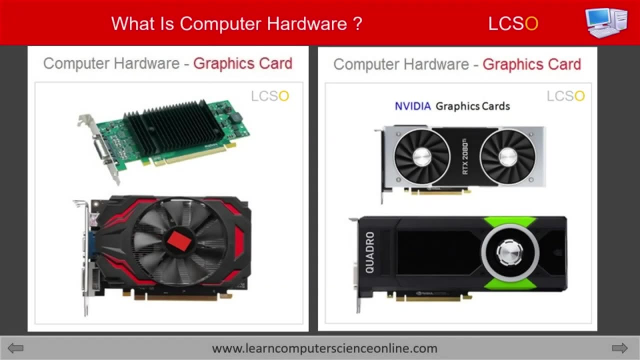 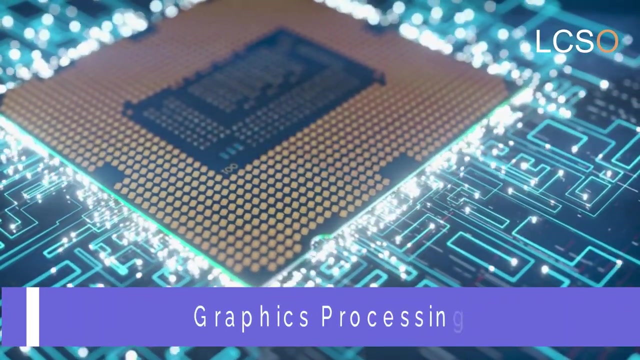 motherboard. The RAM modules are installed and mounted into the memory slots provided on the system motherboard. The RAM modules are also commonly referred to as DIMM. The next important hardware component on our list is called a graphics card. The graphics card is equipped with a dedicated microprocessor which provides adequate processing power to independently handle. 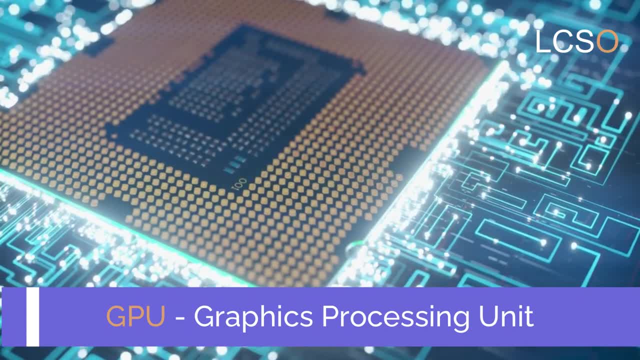 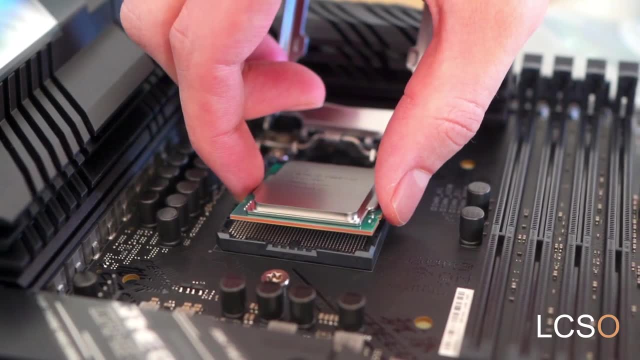 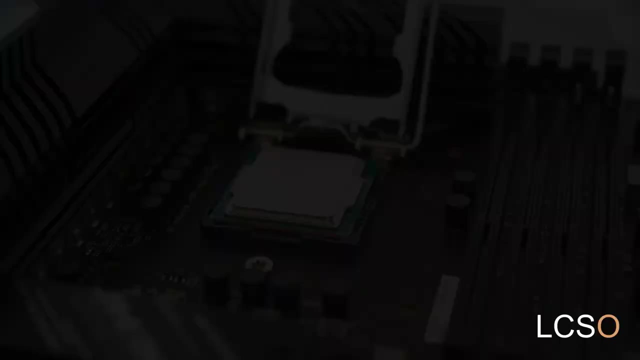 the graphics processing function. High-end computers are equipped with a separate graphics card with a dedicated processor called a graphics processing unit, GPU. High-performance computers are mainly used for some high-end jobs such as video editing, computer graphics or simply for playing any high-end video games. The graphics card, 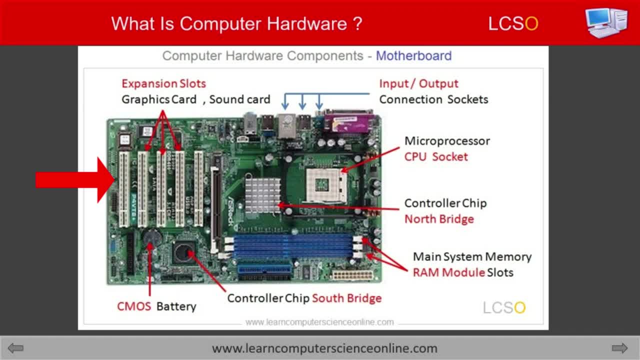 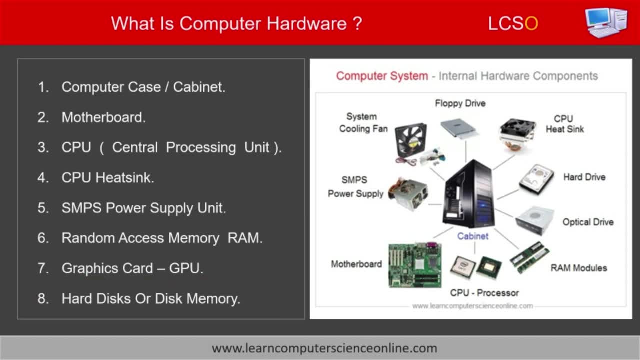 significantly improves the user experience and the quality of the graphics rendered by the computer system. Let us move on to the next hardware component on our list, that is, secondary memory, called the disk memory or a hard disk. The hard drive or a disk memory is used to store the data. 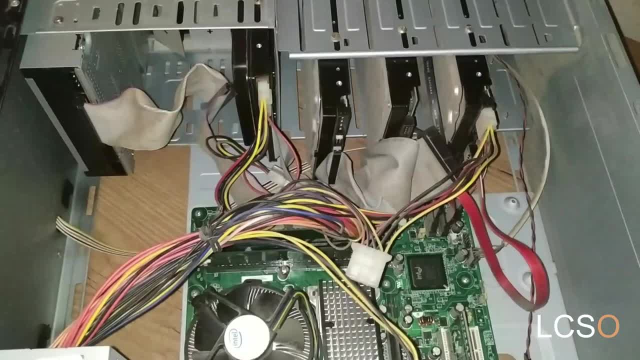 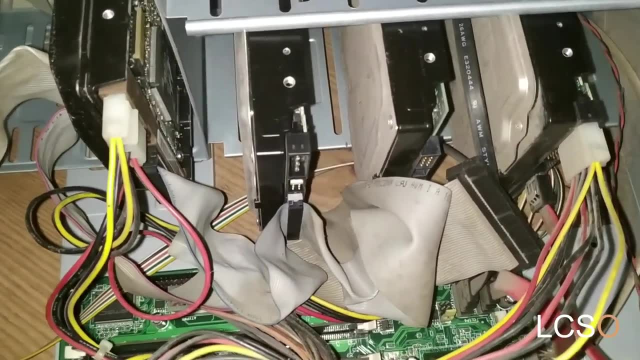 the disk Hard drive hardware is also using the term SDS, which means self-serteving memory or crunching memory, or just non-shutter memory, which is a dual memory that購man worship as if it wereorge or anahanfinal memory. The hard diskivolving system consists of the: 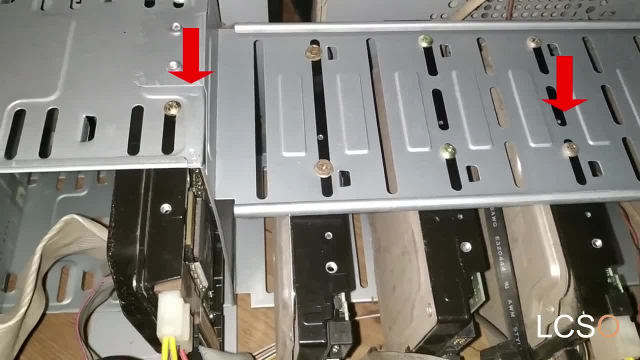 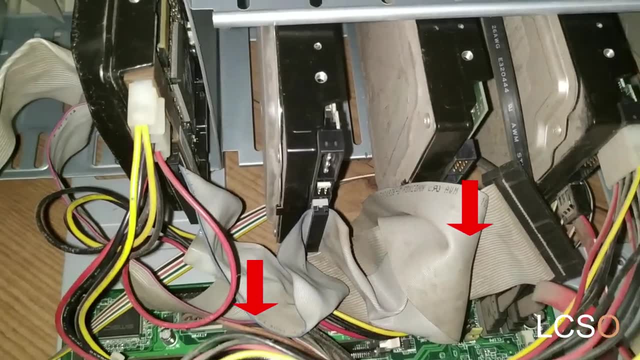 hard drive and is mainly available as a storage memory: Tabloid 128.. cosas of memory are constantly being applied to hard drives. EST denotes the 저는Gebl으니까 Elle, bathroom memory and wishing I had the accession use cases in case I really need it. The hard drive記는 SDS in the memory of a called. 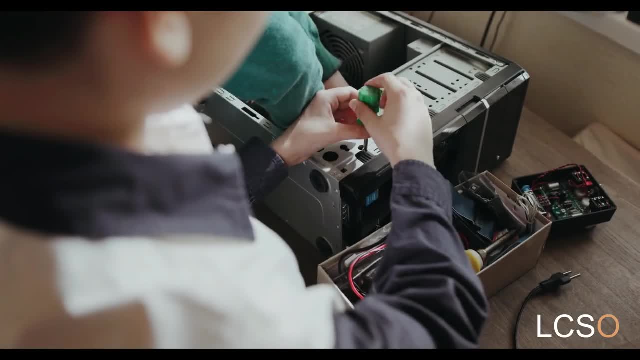 memory它 awesomey called a secondary memory- and it is managed by the operating system. The hard drive is mounted into specific slots present in the computer case. The computer case promises multiple unit. The user can also connect the external hard disk through any USB port. The hard disk. 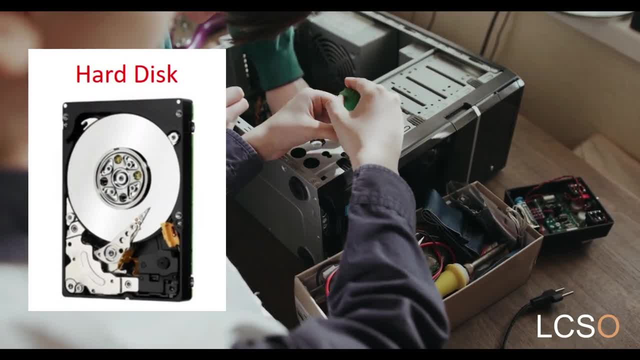 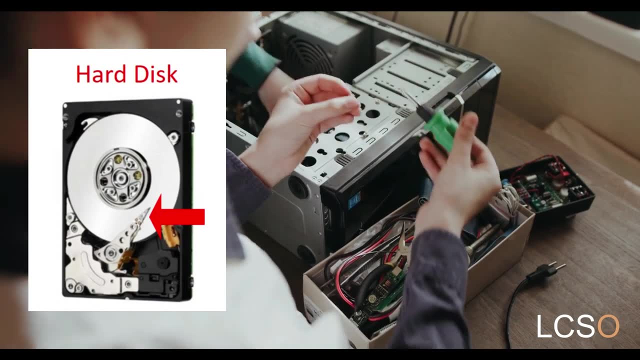 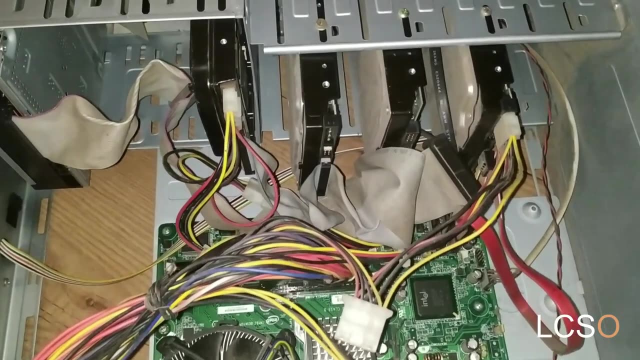 runs on a mechanical moving parts which consist of number of rotating storage disks and a mechanical head which reads and writes the data. The moving parts into the hard disks makes it prone for mechanical failure after prolonged usage. The hard disk technology is being replaced by 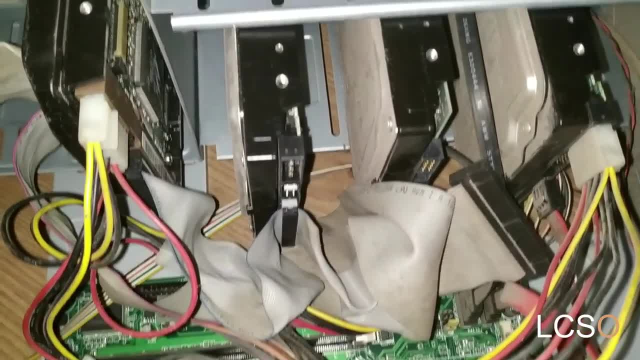 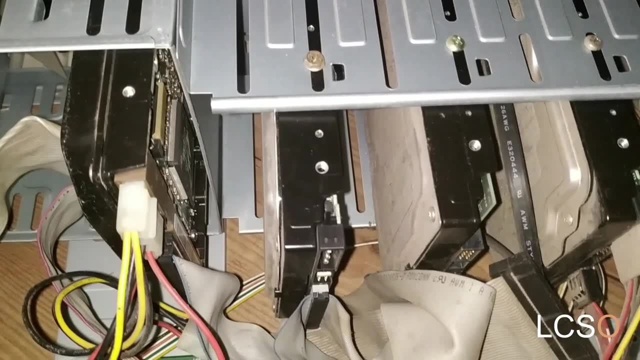 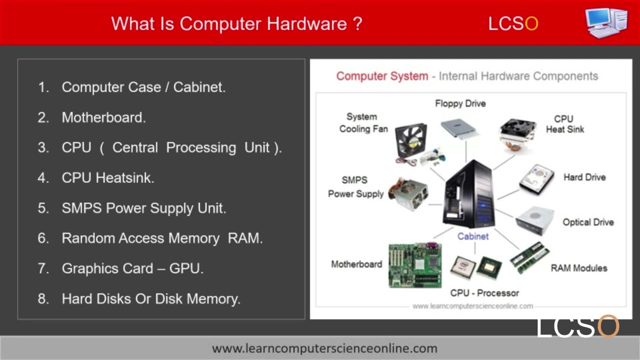 solid-state drive disks, called SSD drives. However, SSD disks are very expensive options at the moment and therefore the hard disk is still being used extensively for data storage. All right, so far we have covered all the major hardware components and its functions. 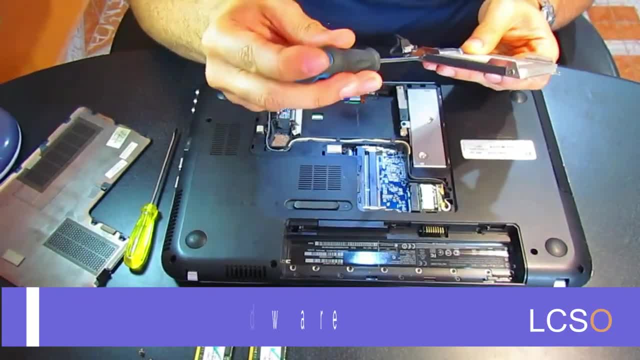 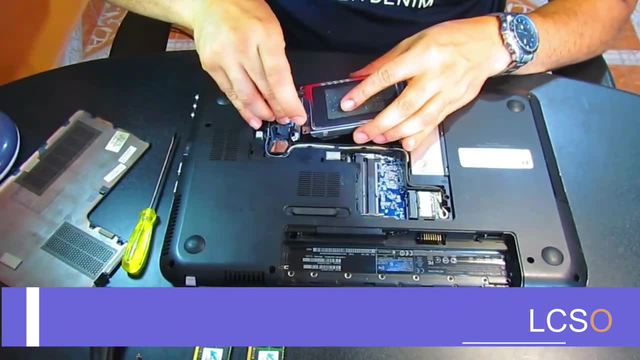 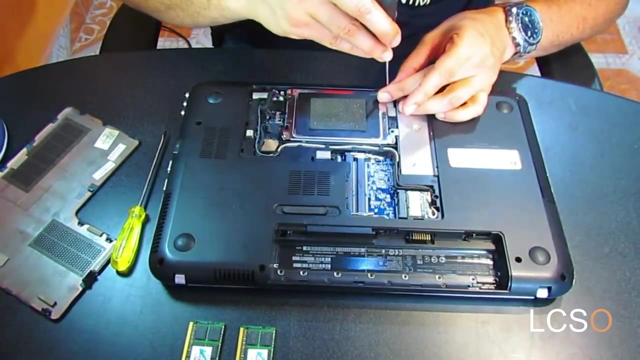 Let us now briefly cover a final note on the laptop hardware components. The hardware architecture for the laptops have gone through a major technological change in terms of motherboard design and integration of other hardware components, especially for slim range of laptops, But in terms of functionality and the system architecture. 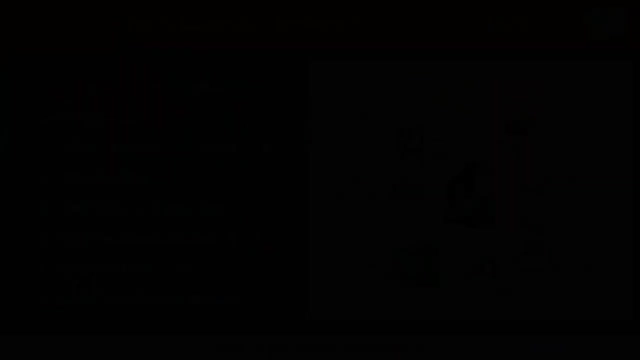 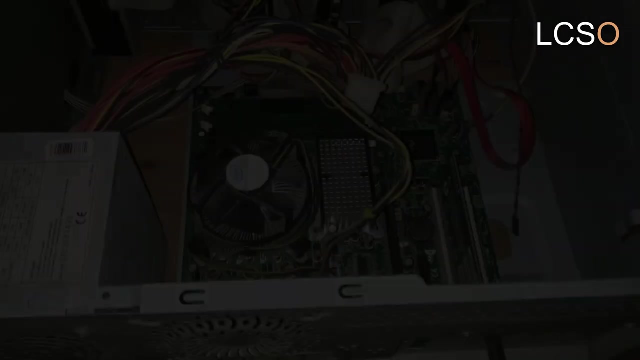 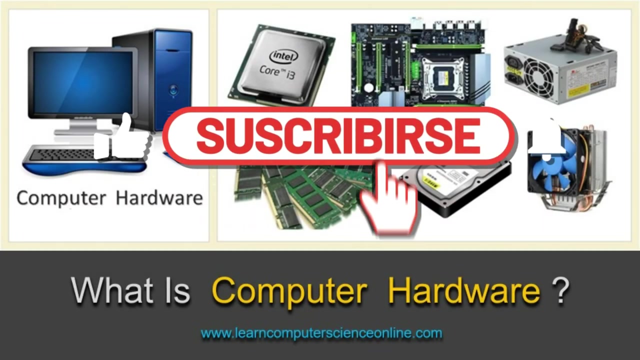 the laptop hardware components also works are same. Okay, so let us do a quick recap. So far, we have discussed what is computer hardware, different types of hardware components used in the computer and its functions. All right, so that brings to the end of this. 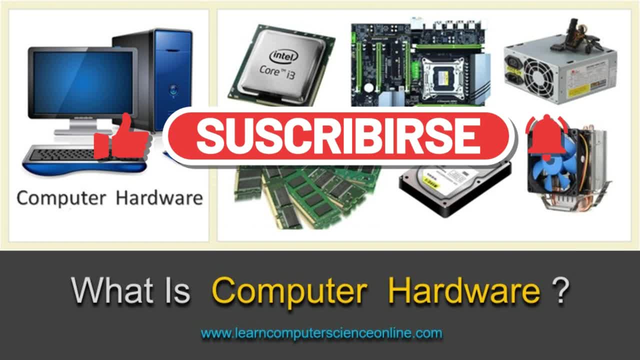 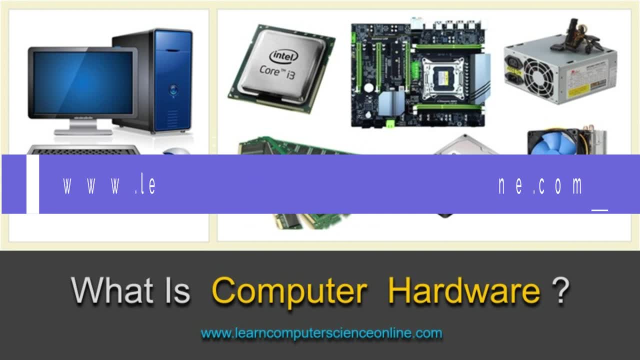 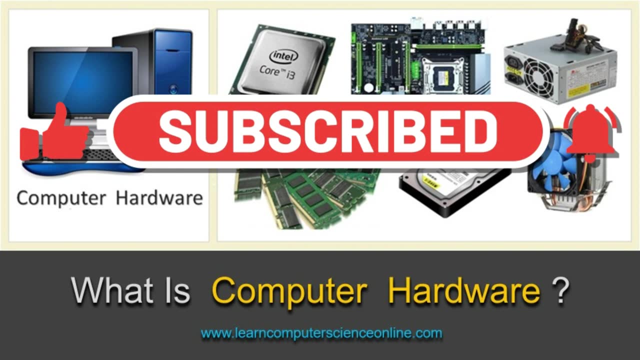 tutorial: What is computer hardware and computer organization and architecture. Please visit our website learncomputerscienceonlinecom for detailed article on computer hardware. If you have liked this video, then please give us a thumbs up And consider subscribing to this channel. Thanks for watching. 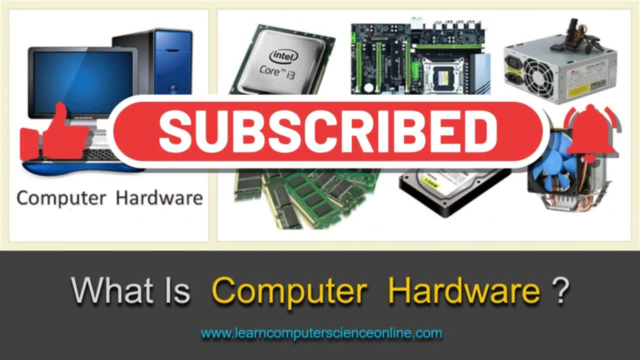 and I will see you soon with another interesting computer science tutorial.